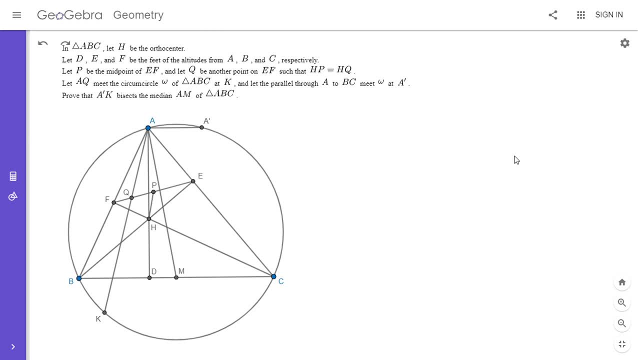 Hi everyone. it's Michael, So I have a staggering problem for you all today. This one was sent to me by one of the viewers of my channel and it was his own problem, So he created it himself and I found it to be quite challenging. So if you'd like to try to solve it, 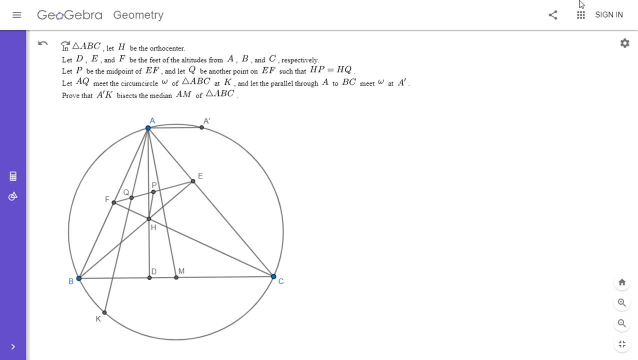 feel free to pause the video. All right, so I'm going to go over the solution. So we have a triangle: ABC, H is the orthocenter, D, E and F are the feet of the altitudes from A, B and C. 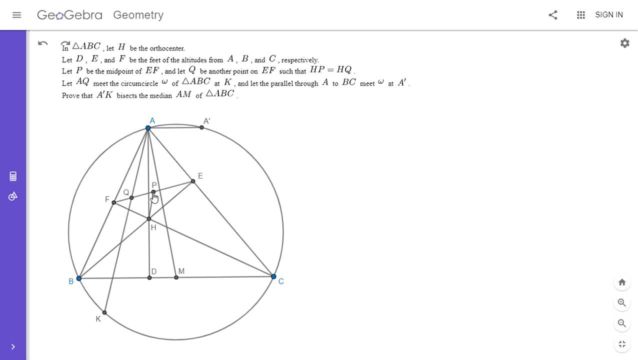 We then let P be the midpoint of EF and Q is another point on EF, such that HP is equal to HQ. AQ meets the circumcircle of ABC at K, and A' is the intersection of the parallel through A to BC with the circumcircle, And we want to show that A'K bisects the median AM of. 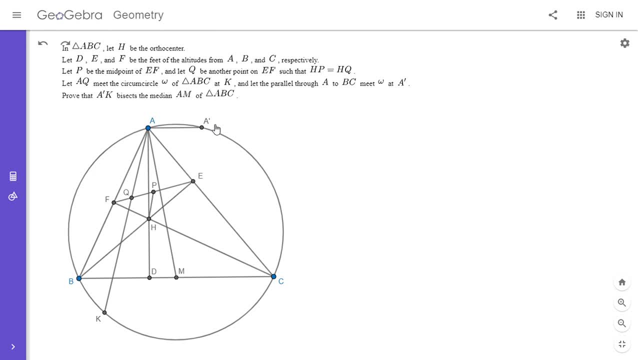 ABC. So I haven't drawn the segment A'K. but if we did draw it, then the problem says: to show that it bisects AM where M is the midpoint of BC. All right, so how do we get started here? 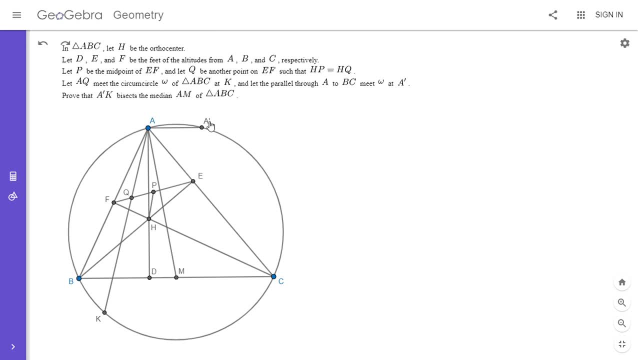 Well. so one thing I thought is that if we want to show A'K bisects AM. well, the diagonals of a parallelogram bisect each other. So an idea I had was to reflect point M across D, So I'm going to call that M' And then, if we can show that A, A' M, M' is a. 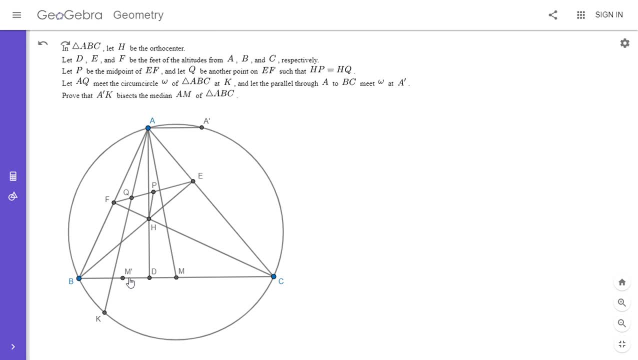 parallelogram, which I'll do in just a second. then we know that A'M' bisects AM, So the problem is equivalent to showing that A', M' and K are collinear, which looks like it might be a little. 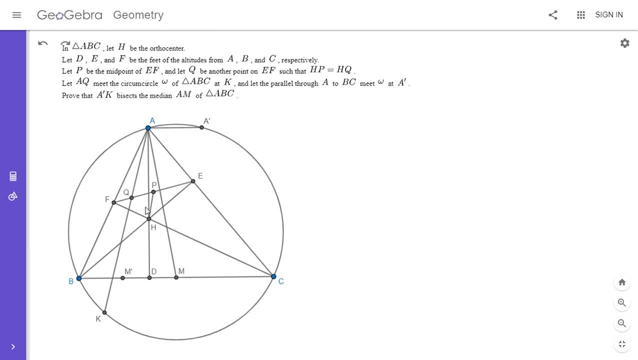 easier, So I'm going to go with that approach. So it's not hard to show that A'K bisects AM, but A A' M, M' is a parallelogram, So I'm going to do it right here. 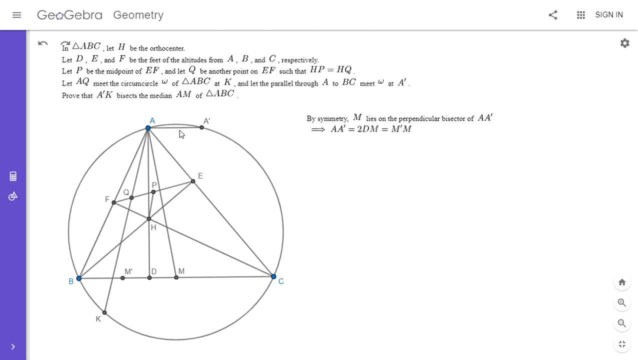 So it's clear that M lies on the perpendicular bisector of A- A' That's true because A- A' C- B is an isosceles trapezoid, And so A- A' is 2DM, which is M'M, because M' is the reflection. 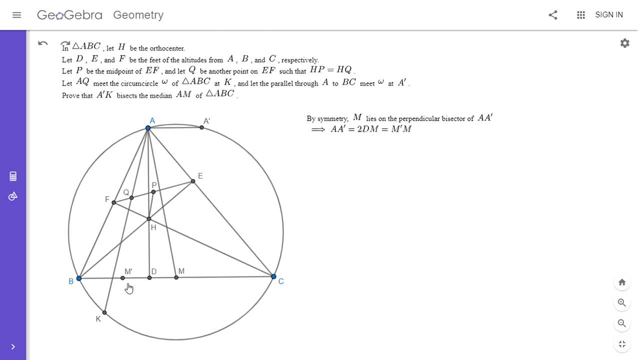 of M over point D. That's how I defined it, And so if A, A' is equal to M'M and at the same time, so those segments are equal in length and they're also parallel. So I'm going to write this out. So if you have two segments that are 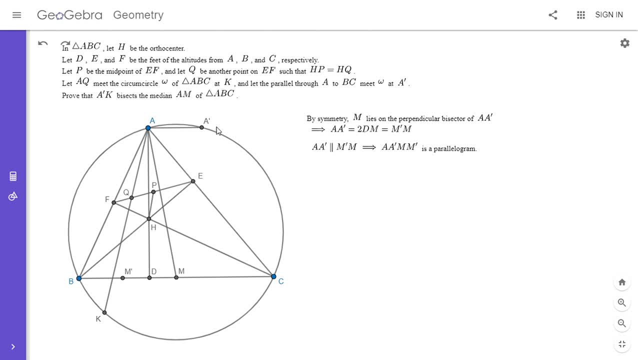 the same length and they're parallel, then they form a parallelogram. So A A' M, M' is a parallelogram And so its diagonals bisect each other. So really we want to show that A' M' and 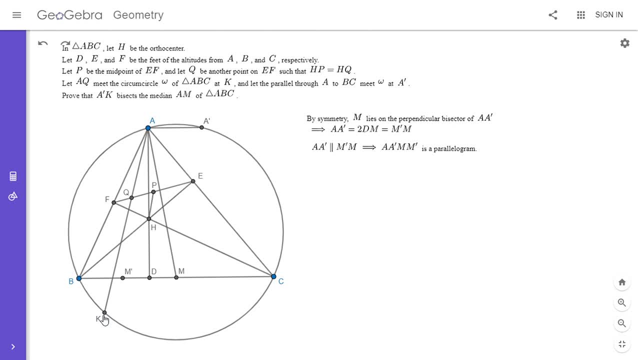 K are collinear, That would solve the problem. So if you have two segments that are the same length, that would solve the problem All right. So the next thing I noticed was so: first B, F, E, C is: 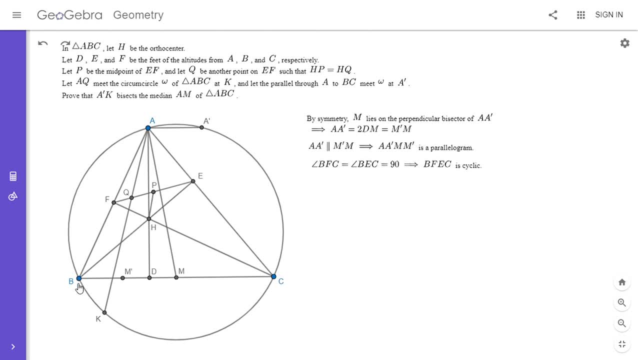 a cyclic quadrilateral, So that's a well-known fact. That's true because angle B F C is equal to angle B E C, which are both 90 degrees. So B F E C is cyclic, And so that means triangle. 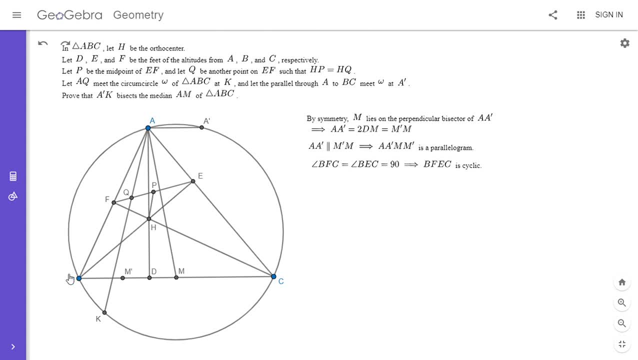 F, H, E is similar to triangle B, H, C And that looks like it could be useful, because P is the point of E, F and M is the midpoint of B, C. So P and M are basically corresponding points in those. 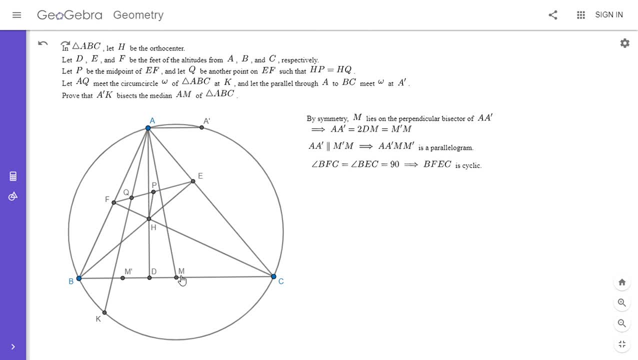 two similar triangles, But the thing is they're oriented differently, So it's kind of like one is like the reflection of the other. Of course you'd have to scale it also, But I wanted to try to make them oriented the same way, And you'll see why in just a second. So first I'm going to state what I. 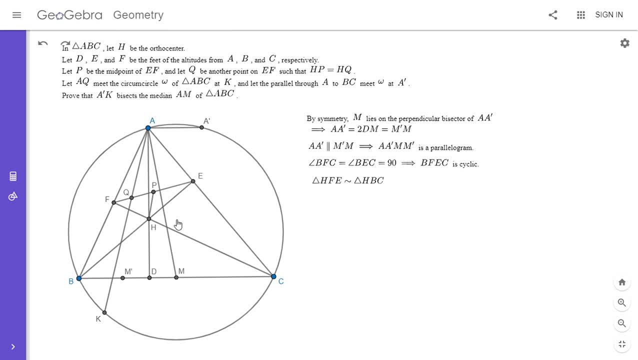 So triangle H F- E is similar to triangle H B- C. That's very easy to see. It's easy to show that the angles are equal, Because angle F E- B is equal to angle F C- B And angle E F- C is equal. 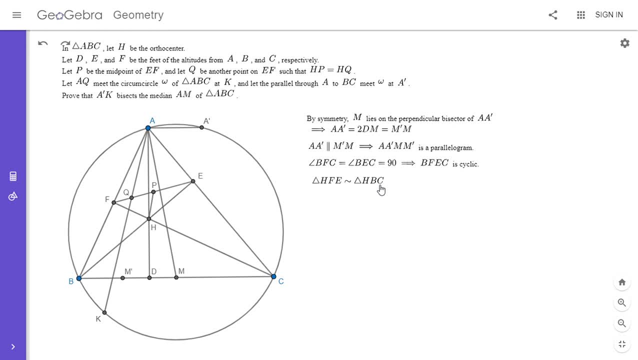 to angle E, B, C. Okay, So this is a well-known fact, But now I'm going to use the fact about the orthocenter that when you reflect it over a side, it lies on the circumcircle. So if we let H 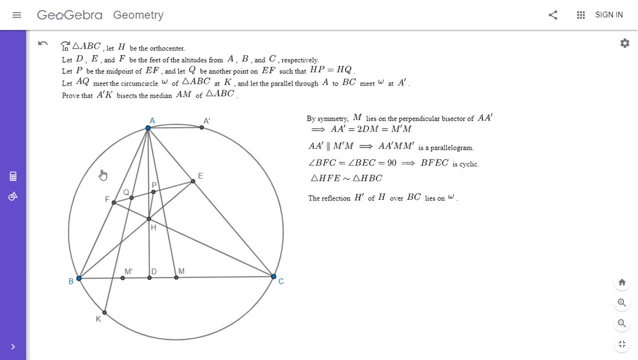 be the reflection of H over B, C, then H prime lies on the circle omega. All right, And if that's true I'm going to draw in a couple more lines. That means the triangle B, H, C is congruent to. 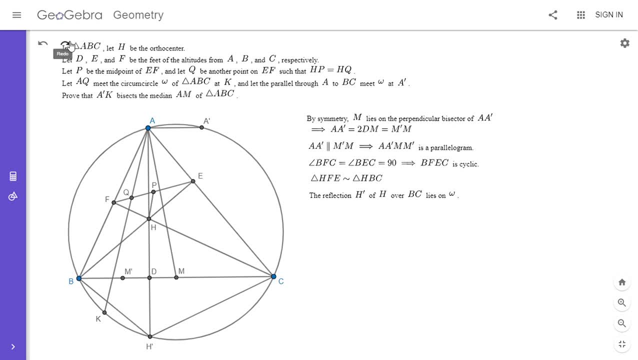 B H prime C. Okay, So we actually have the following. So triangle B H C: it's congruent to B H C, which is similar to triangle F H E. So we now have that. 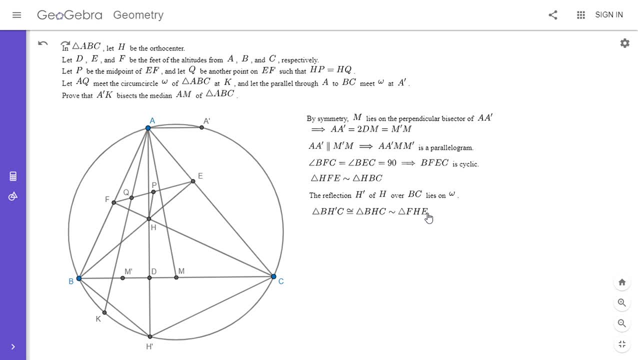 And that means that the first and last triangles have to be similar And they're also oriented the same way, which is going to come in handy, All right. So we have: M corresponds to P in those two triangles, because M is the midpoint of B- C and P is the midpoint of B- F. All right. 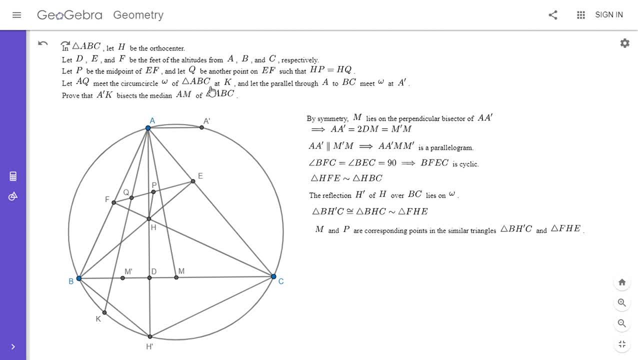 So that looks like it might be helpful, But not only that. here's where we're going to use the. We know that H P equals H Q, but it's also very easy to see that H prime M is equal to H prime M. 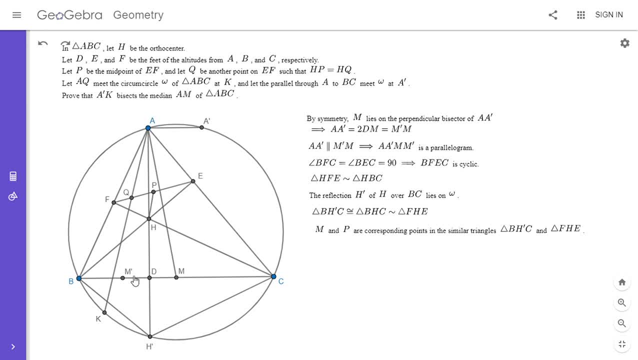 prime. That's obvious because M prime is the reflection of M over point D, So I'm going to write this out. So since H P is equal to H Q and H prime M is equal to H prime M prime, basically that means in these two similar triangles, M prime and Q are corresponding. 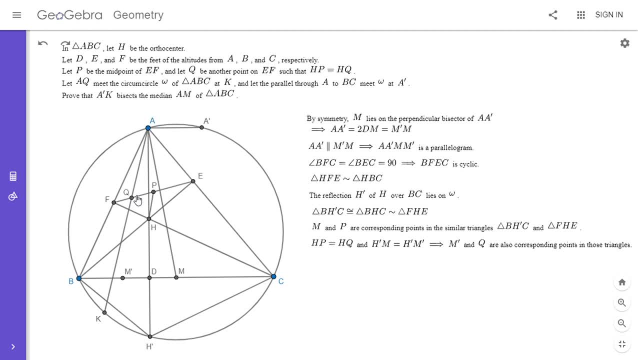 points. So basically, M, prime and Q break up the segments B, C and F? E in the same ratio. All right, And then I'm going to notice one more thing. Not only are these two triangles similar- B? H prime C and F? H- E- but the whole quadrilateral A, B H, prime C- is similar. 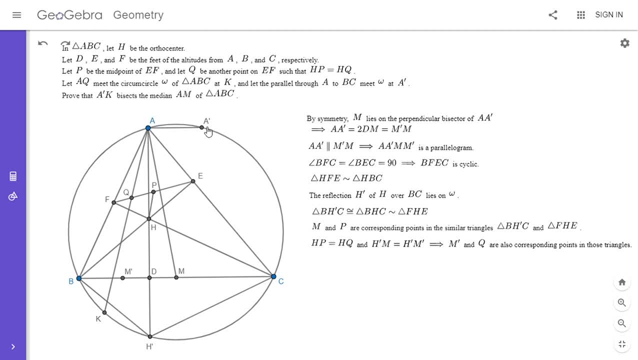 to the quadrilateral. I'm sorry, the whole quadrilateral- A, prime H, prime C- is similar to A, F, H, E, So I'm going to show this here. Some of you will just recognize this from properties of spiral similarities, but I'm just going to write. 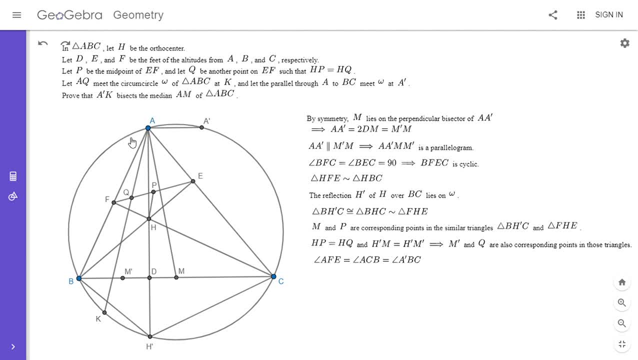 out the full proof, just for completeness. So we have: angle A F, E is equal to angle A C, B. That's true because B, F, E, C is cyclic And angle A C- B is equal to angle A, prime B, C. 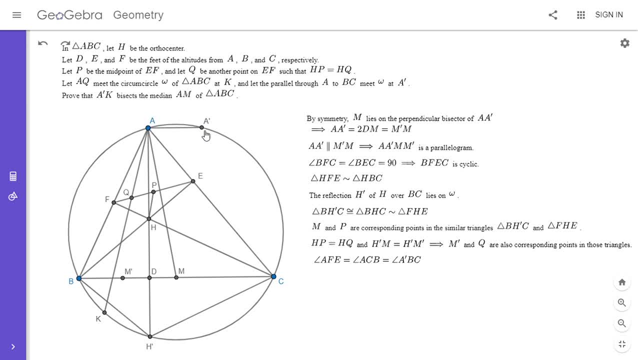 That's true by symmetry, Because A, A prime C B is an isosceles trapezoid. So if you look at the two triangles, A F E and A prime B C, this shows that one of the pairs of angles is the same. 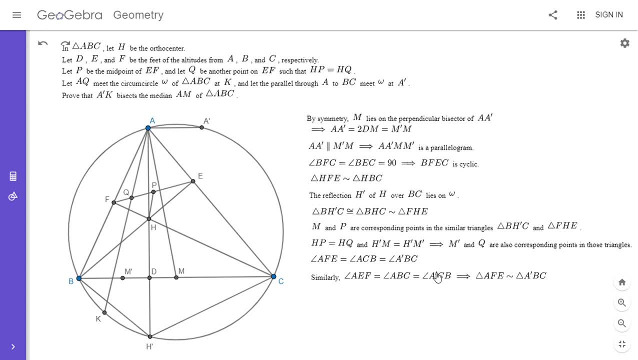 And we can use the exact same argument for the other pair of angles. And so triangles A, F, E and A prime B, C have to be similar. And so basically that means that the whole quadrilateral A, F, H, E and A prime B H, prime C have to be similar. All right, Because if you have two pairs, 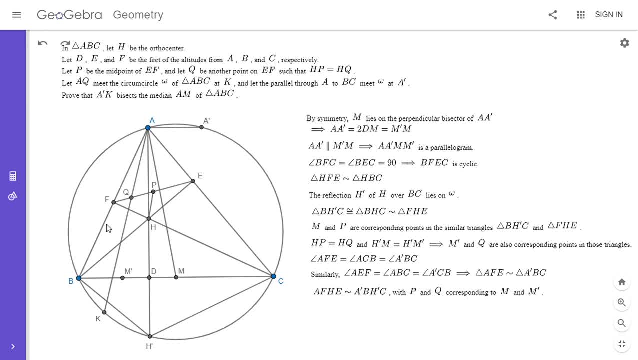 of similar triangles. so B, H prime C is similar to F, H, E, And also A prime B C is similar to A, F, E. So that means those quadrilaterals as a whole have to be similar, And we mentioned that. 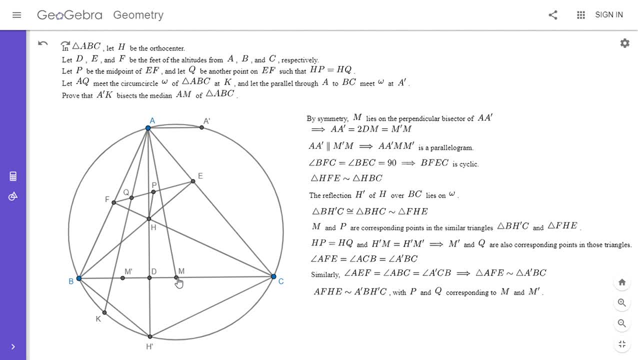 P, F, E and A prime, B, C have to be similar, And so if you have two pairs of similar triangles, A corresponds to point M, because they're both midpoints of a diagonal in that quadrilateral, And Q has to correspond to point M prime. So this gives us a lot of information, And now we're. 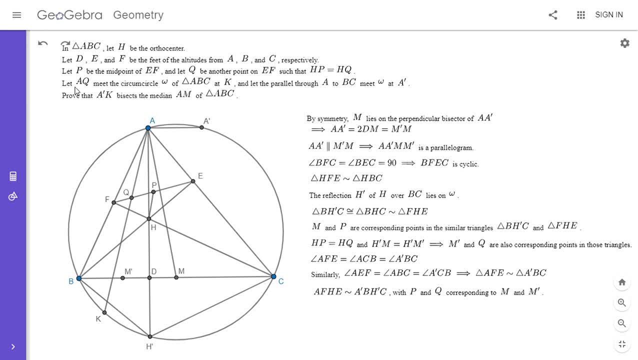 really close to solving the problem, All right. So now I'm going to use all the information I have to do an angle chase that'll show that A prime, M prime and K are collinear. All right, Let's see, would that? 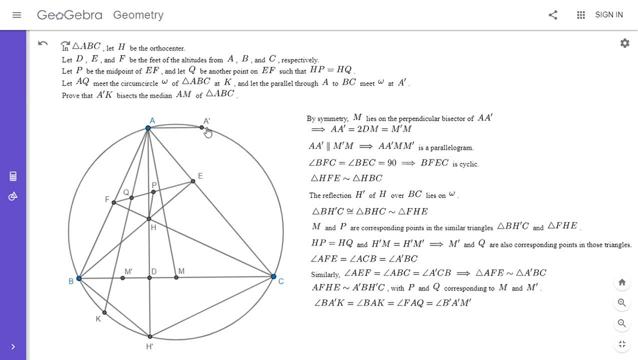 So we have. so one way to do that is to show that angle BA prime K is equal to angle BA prime M. So I'm going to show you here how I do that. So we have: angle BA prime K is equal to angle BAK.